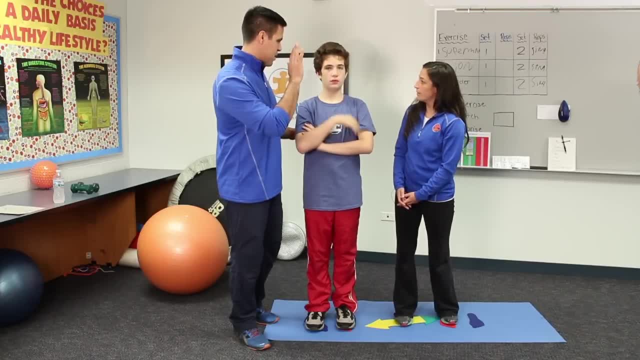 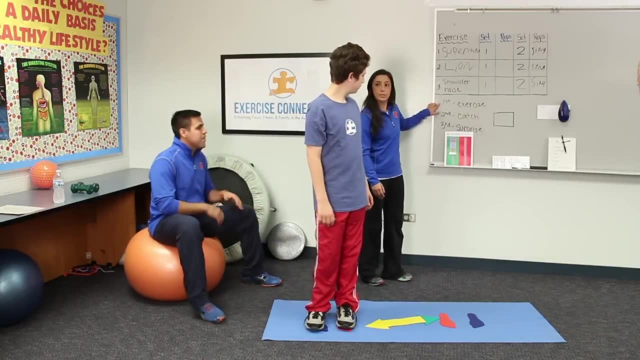 Yes, Okay, All right, I'm going to step away, Dylan. I want to see what you've been doing. You ready? All right, You want to coach Ashley to go do it. So, Dylan, what are we going to do first? 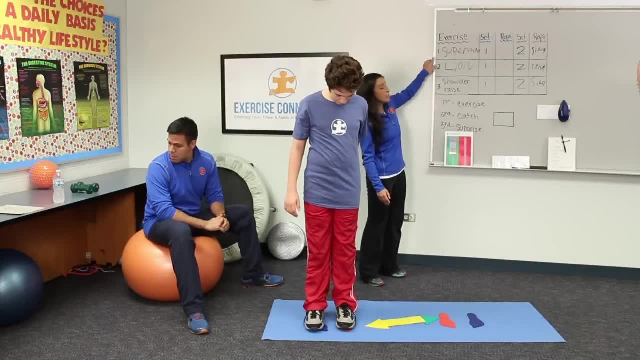 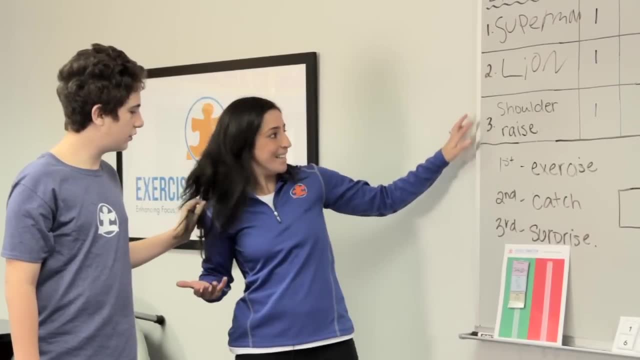 Exercise, Exercise, And thank you for picking the exercises. Thank you, What exercises are we doing, Dylan? What are we going to do first, Superman, Superman, Very good. What are we going to do next Line Line, Shoulder raise And then shoulder raise. And then what are we going to? 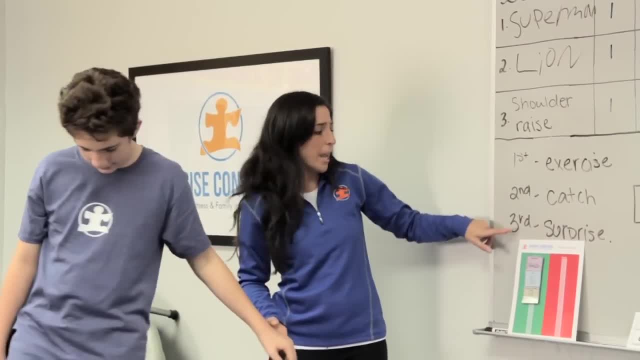 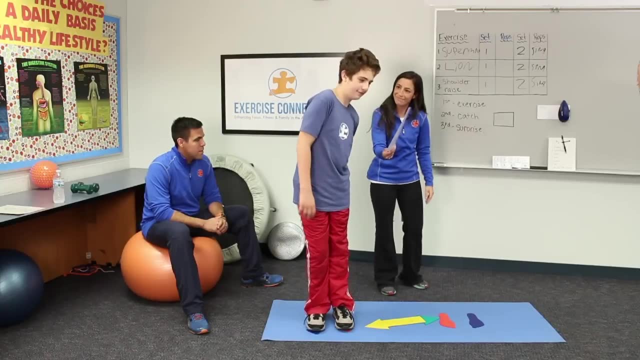 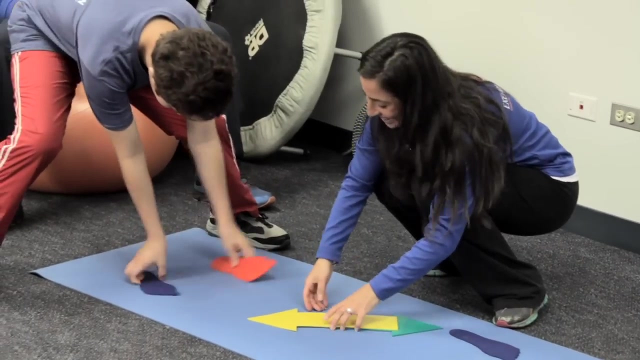 do Surprise Catch, We'll play catch right, And then what are you going to get? Surprise Surprise for your exercise journal. All right, Ready Right here. So she's shown the visual schedule which we've been showing you throughout the series. Very good. 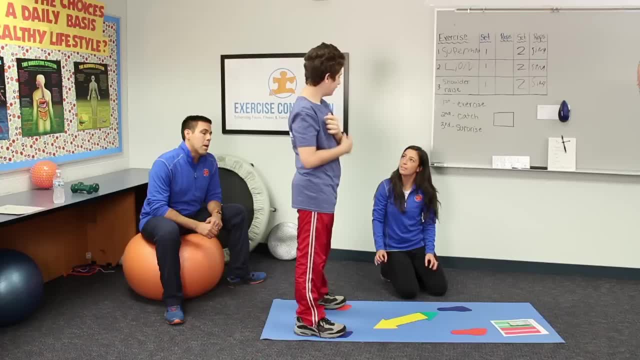 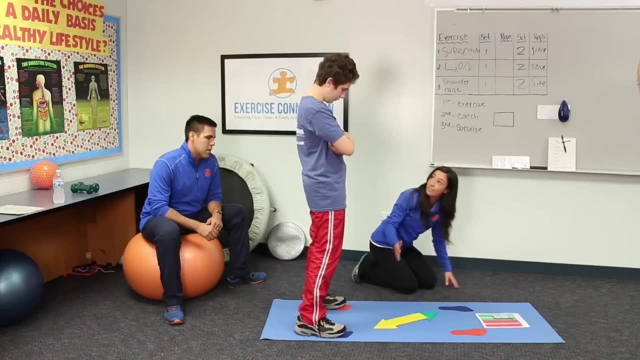 What song are we going to sing? Now? I'm speechless. love bug. Now I'm speechless. love bug, Ready, Love bug. All right, What are we going to do first? Superman? Okay, Dylan, are you going to sing? 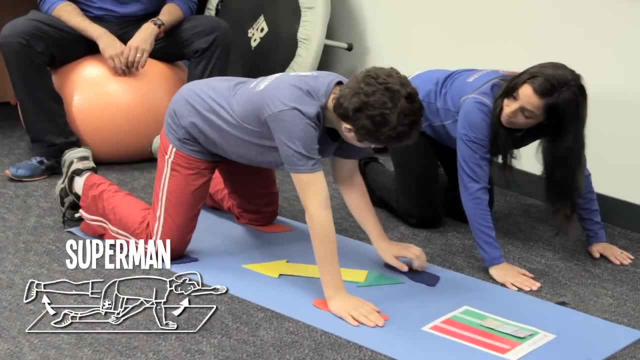 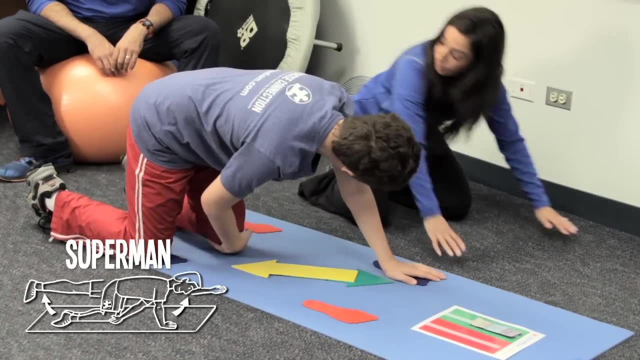 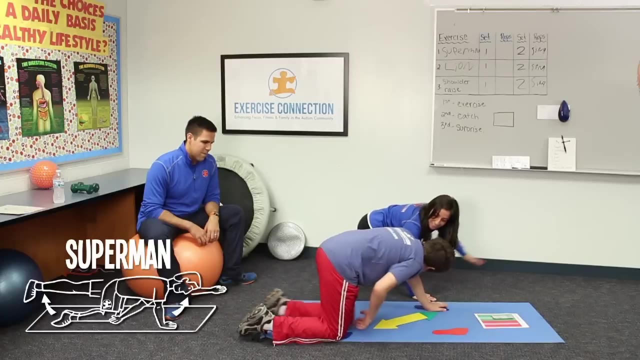 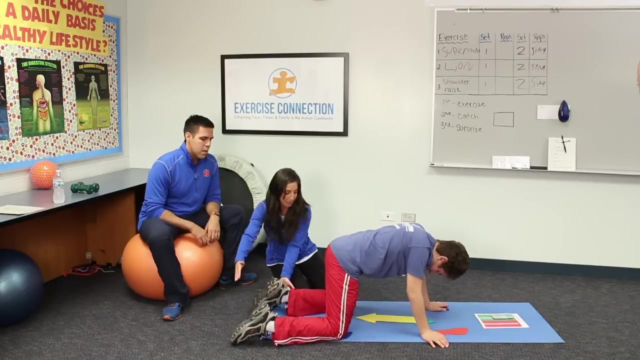 and coach Ashley counts. Yes, Okay, I'll stop counting when you stop singing. Ready Go Good, Good, Keep going Very good. Three, four, five, six, seven, eight, Keep going Good. What Doing both sides of the? 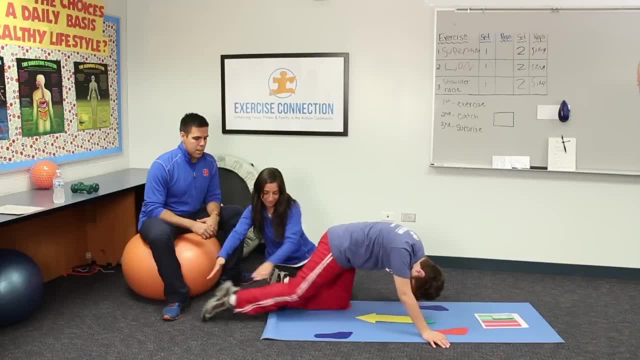 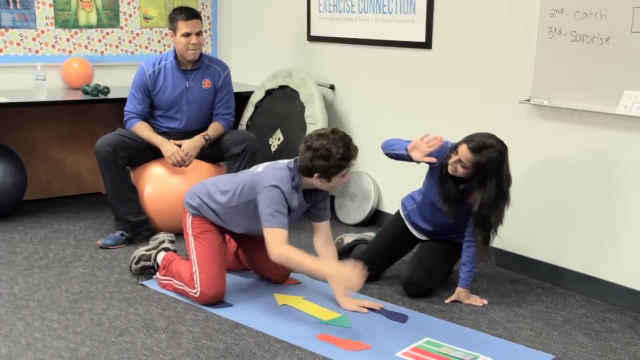 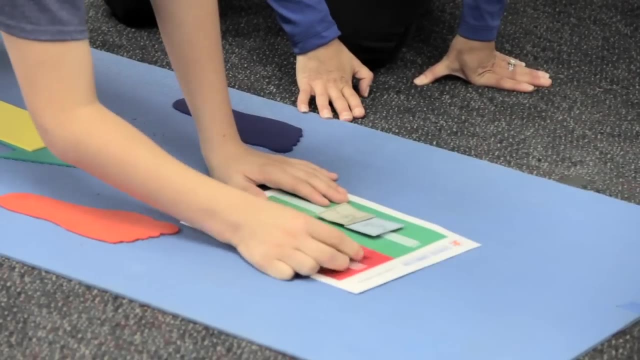 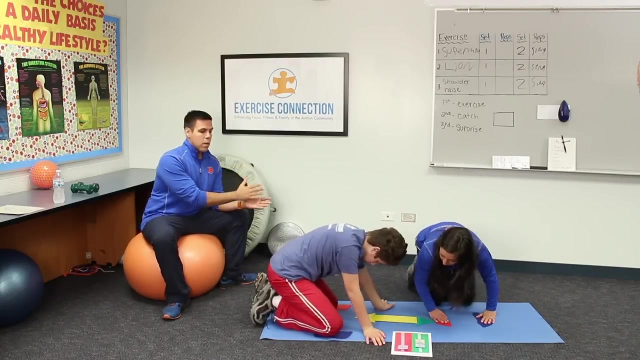 body. This is challenging both sides of the brain. Good Five, six, seven, eight. Very good, Dylan. Thanks, Chad, Did we finish it? Yes, Yes, we did. What's next? Lion, Lion. So, Dylan, move the card from the green, which means go to the. 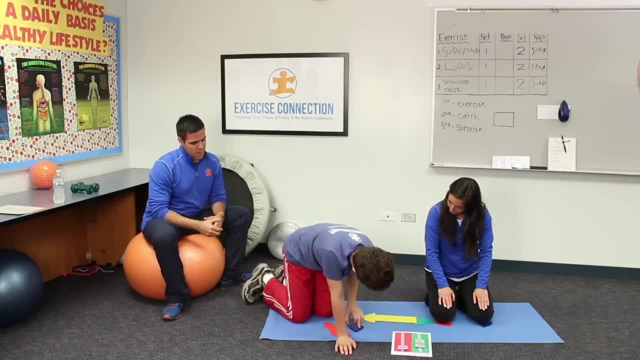 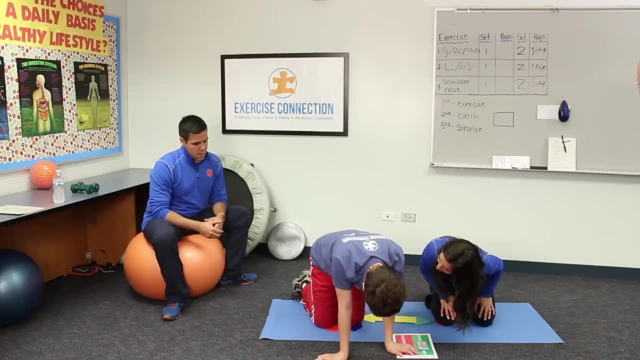 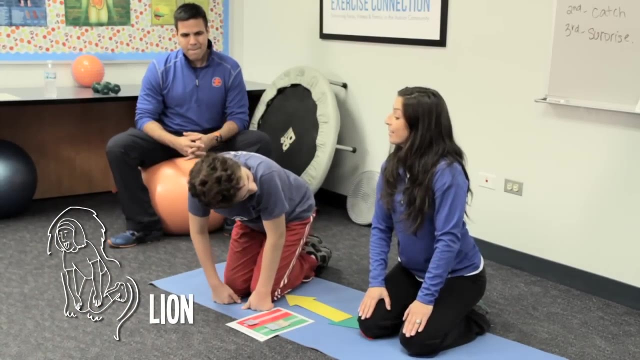 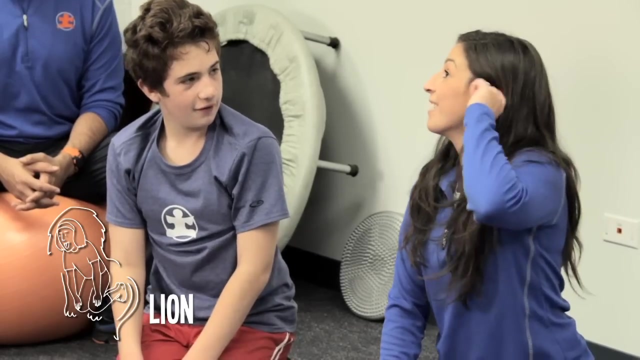 red, which means stop or finish. Nice job, buddy. Yeah, You're good. Thank you for turning the way I am. Can we sing the planet song? Yes, Okay, Ready, Yes, Go. Mercury is number one. Venus is number two. Yes, I'm second. Yes, it's true, Mother Earth is number three. 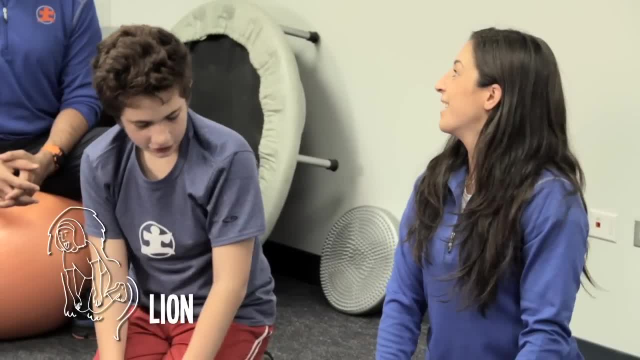 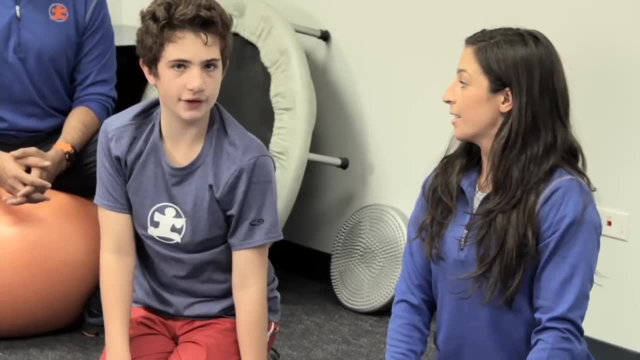 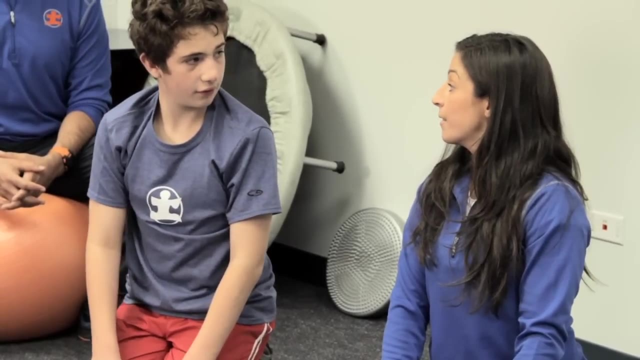 Home is number three. Planet Mars is number four. Can I go for any more? Jupiter is number five- I'm the biggest. Saturn is number six. Uranus is number seven, But it's cold here in the heavens. Neptune is number I wish I'm Don't forget now. dear, I'm very happy. 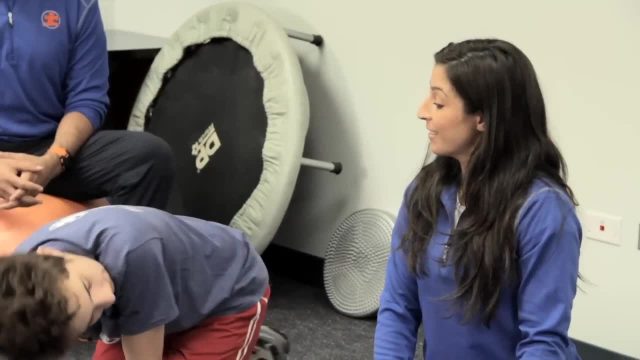 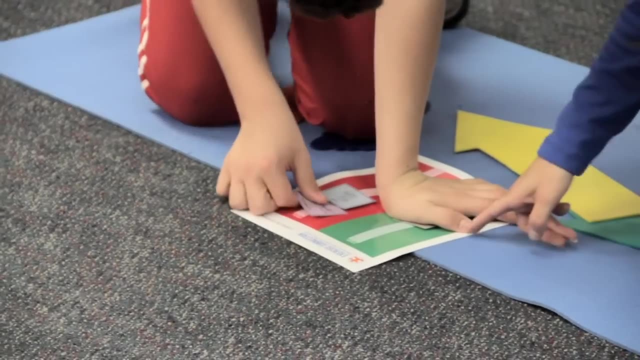 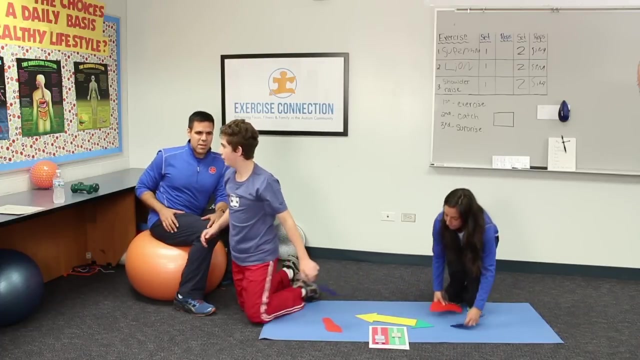 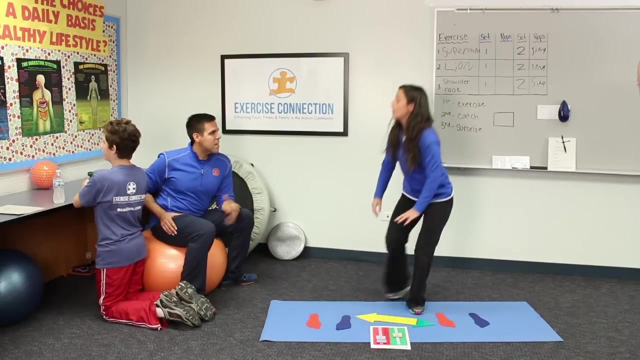 Pluto is number nine. Nice job. Are we done? All right, And what's our last exercise? Double press? Okay, Can you go give the weights? Nice job. So music is the motivator then? Yes, Okay, And do you Anything he wants to With your students? what have you done? Anything. 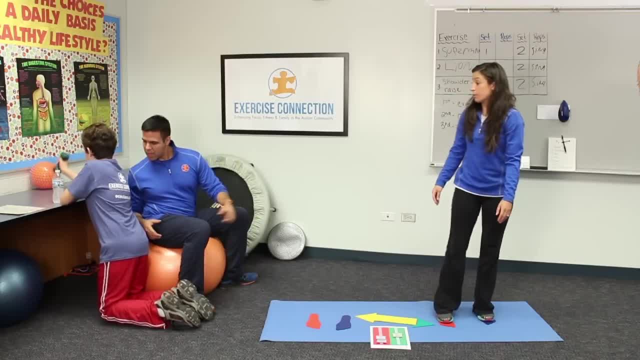 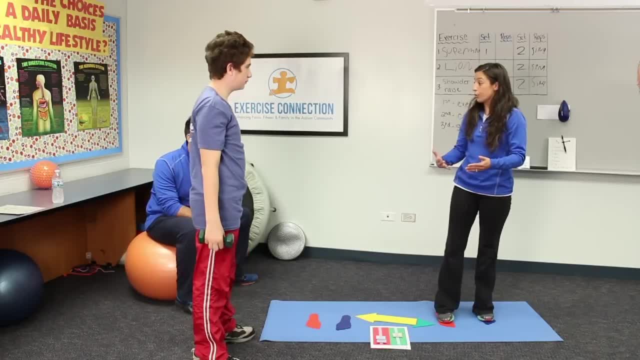 I give them the choice of whether or not I choose maybe the exercise activity or the song Mm-hmm, Or I always give them ownership of their learning and their exercise. so I usually give them that choice. All right, All right Ready. 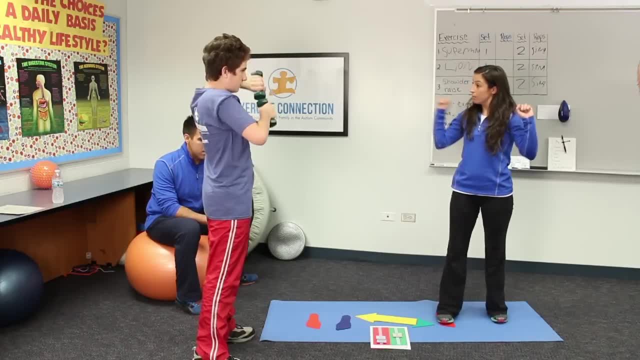 Say it out loud: Are you gonna sing a song or are you gonna count? Sing a song? Okay, what song are you gonna sing? Love Bug, Oh, Love Bug again. All right, Let's the Love Bug Ready Go. 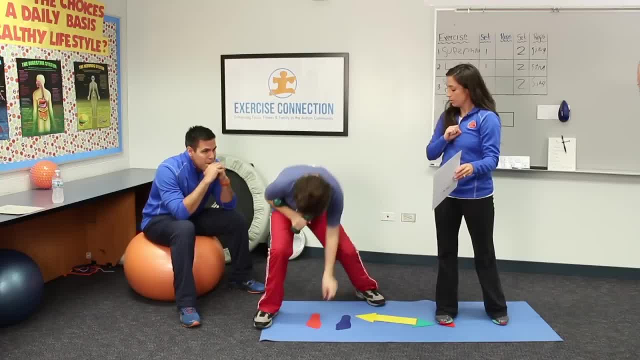 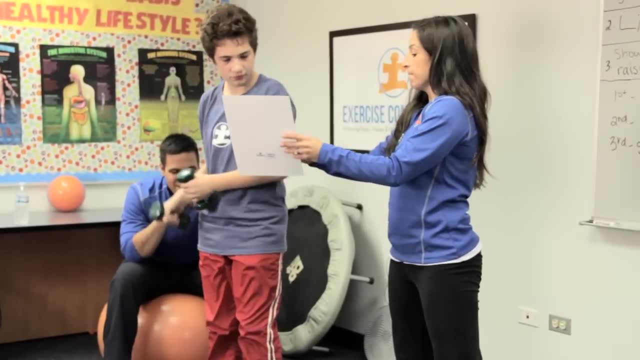 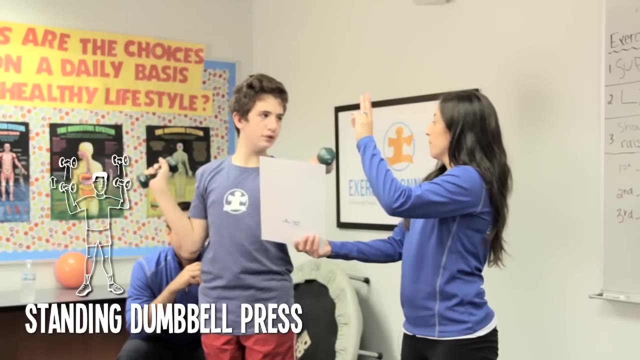 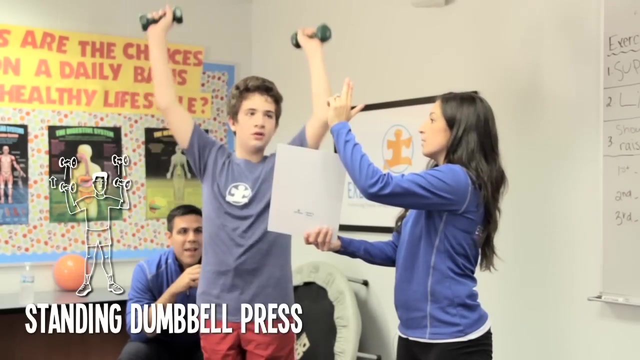 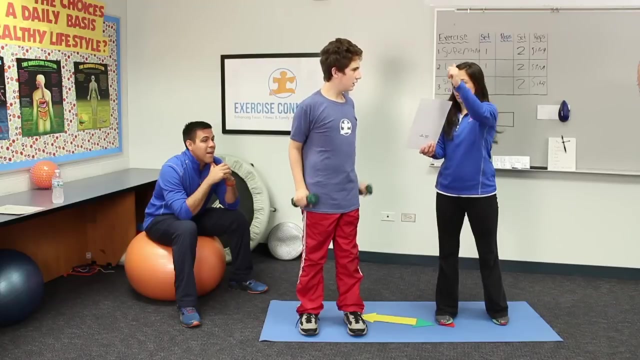 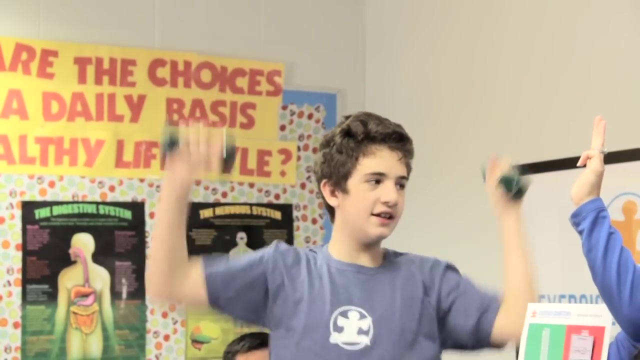 I didn't survive the first time yesterday. I didn't survive the first time. yesterday I found I'm missing a flower. As I close the shopper, Are you done More? Let me say Now: I'm speechless Over the edge of this bright glass. 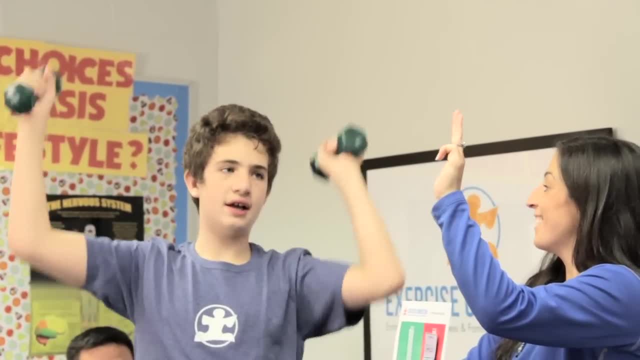 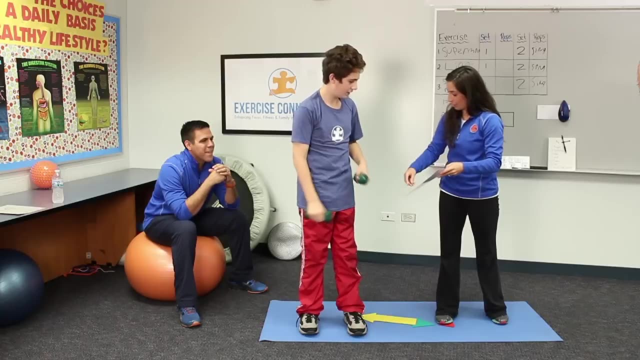 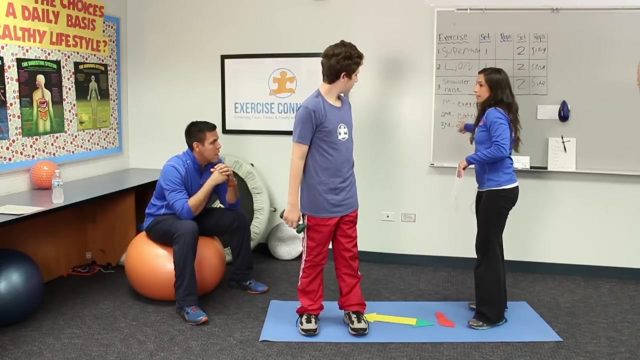 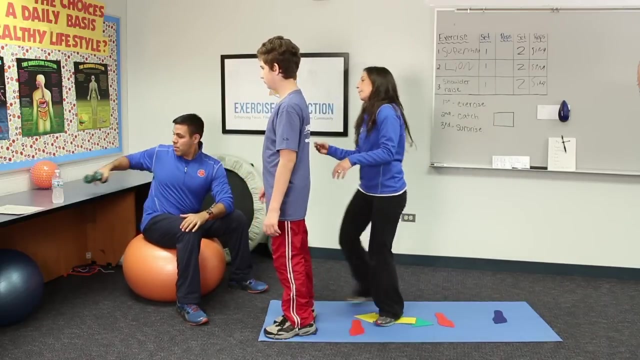 I never thought that I'd catch this. I have it back again Very good. Nice job, Dylan. We'll put this here Very good. What are we going to do next? We'll put this here: Very good. Maybe That's a good shape for the ball. We're good. 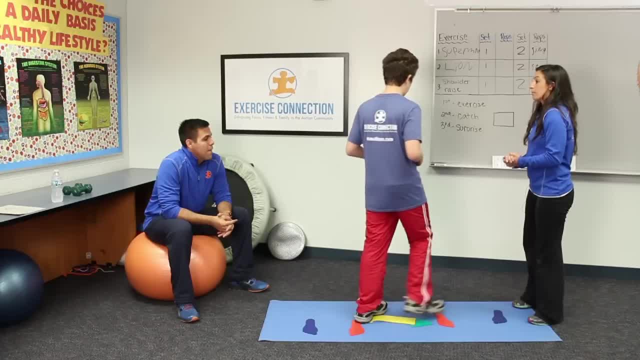 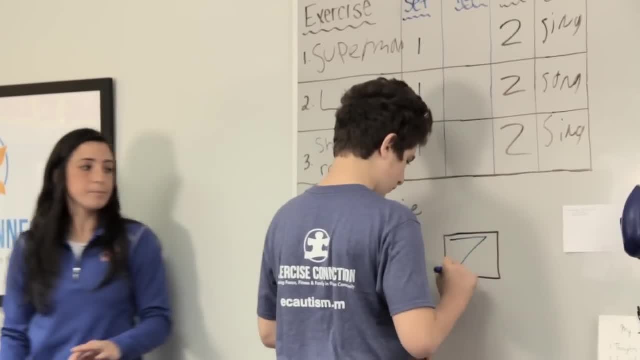 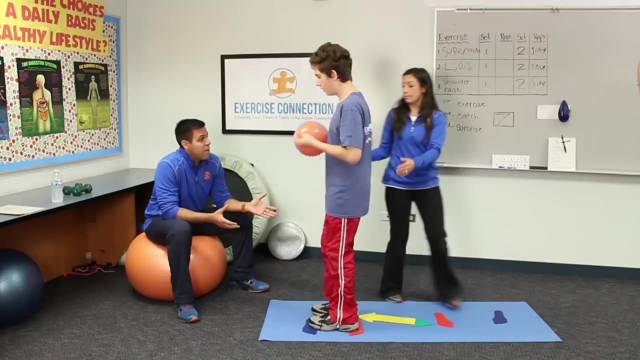 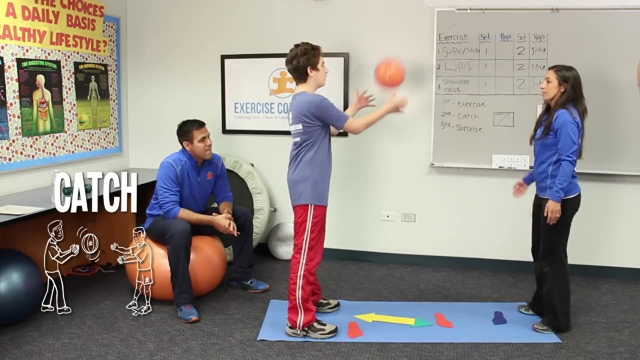 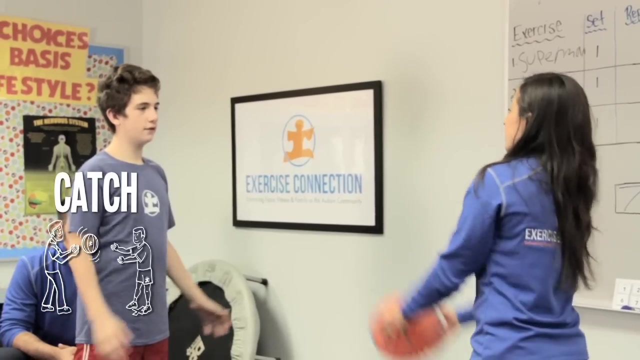 How many catches are we going to do? Seven, Very good. So gross motor. Now you gave him ownership By picking the number And now he just worked a little. five motor, right, Absolutely Awesome, Ready, Ready. One, Two, Three, Three, Two, Four, Five. 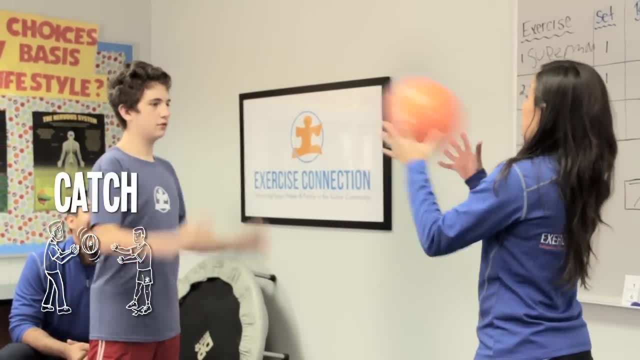 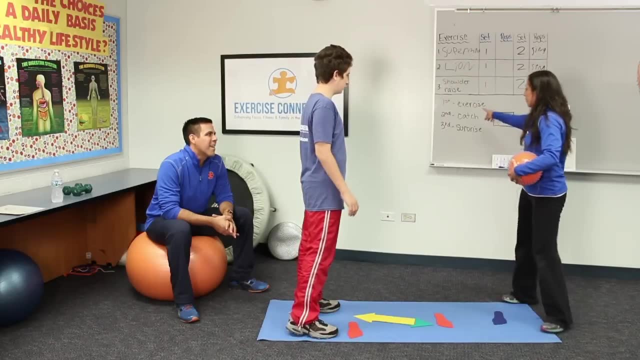 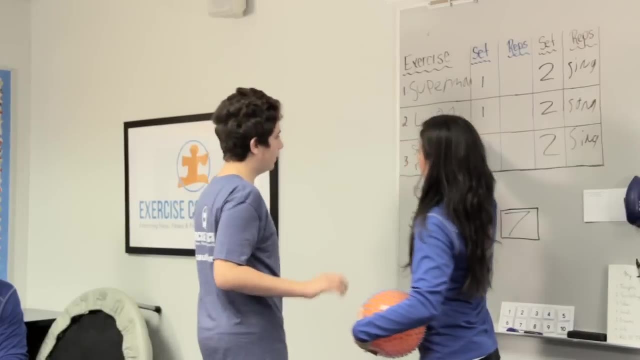 Six, Seven, Eight, Nine, Nine. Should we keep going? Should we still do one more? Yes, Let's do one more. Ten, Ten, Dylan. what did we do? first, Exercise The exercise. What kind of exercise did you do, Superman? Then Lion, You did lion. 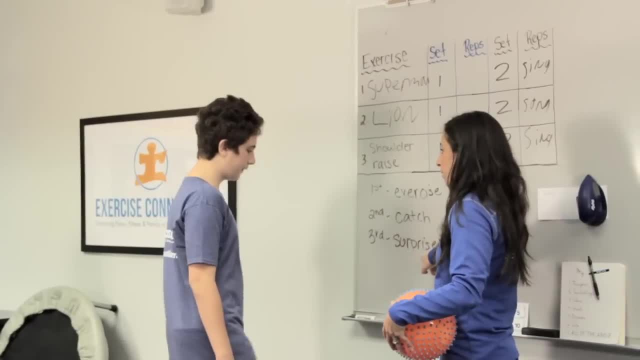 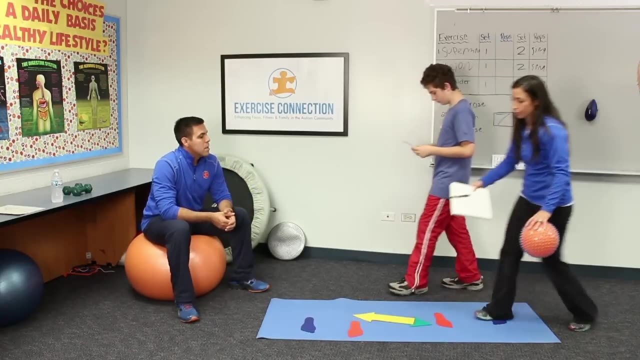 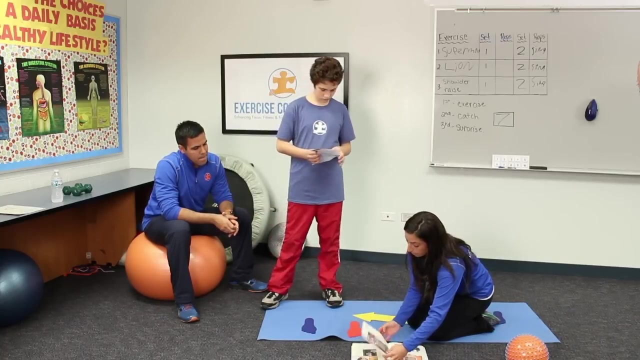 Shoulder raise, Shoulder raise. And then what did we do? Catch, Catch, Surprise, Surprise. Where's your surprise? Yes, Let's bring our exercise journal. So is this something you do after all the routines, After all the exercises? Okay, We work on fine motor skills. 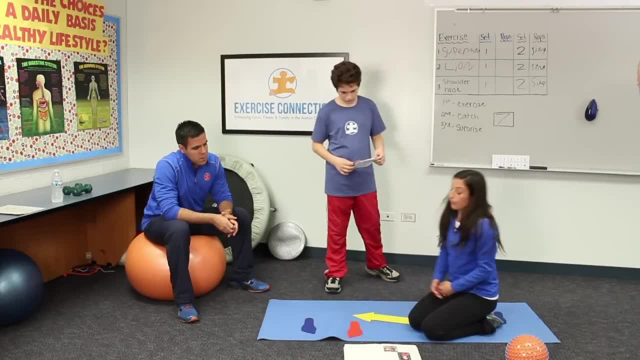 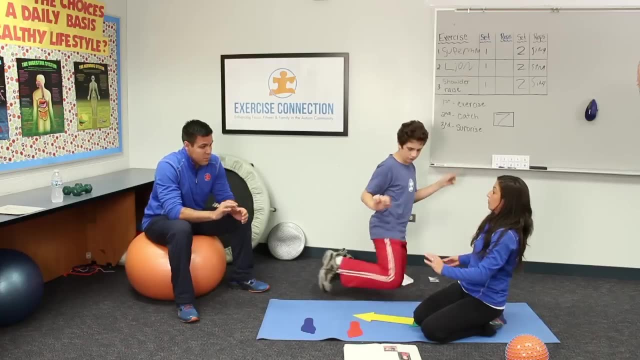 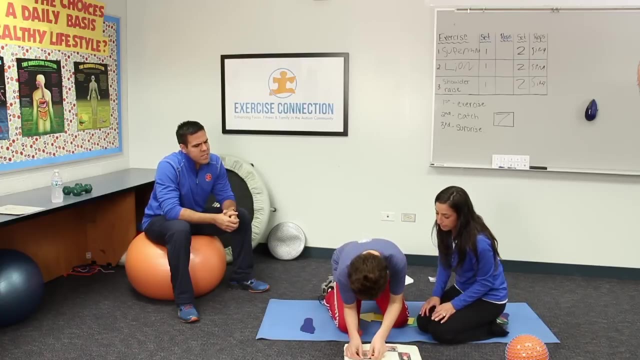 Okay, And we also pick the exercise that he most enjoyed during his exercise class. So working on fine motor, are you saying? you guys are just. This is his writing, His penmanship, His writing, his penmanship. Okay, Look at that. Good, And what's? 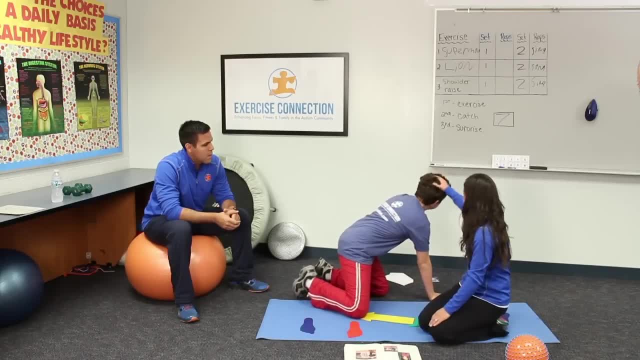 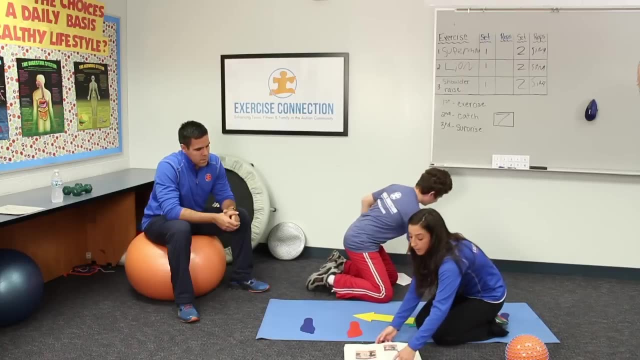 They may not have seen that, but what's he? Ow, Ow, Oh, Okay, You all right. So that's a picture of him exercising. That's a picture of Here's the mirror. It never fails. It makes me want to. When it comes, it won't no more. 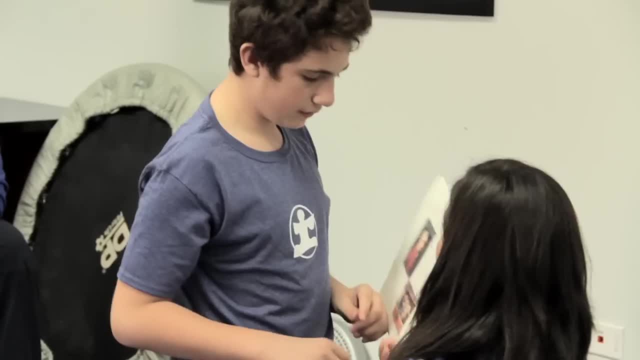 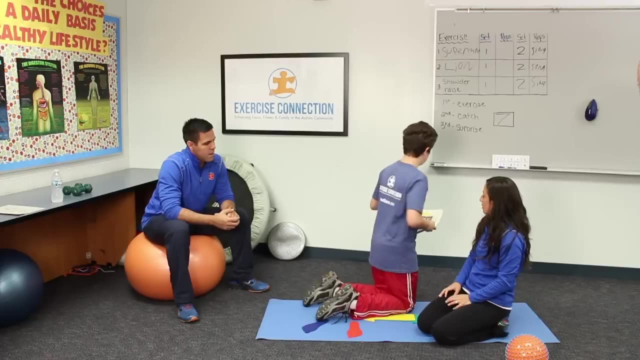 No, What is this? a picture of A guitar? What is this? a picture of Dylan? Dylan what? Exercising? This is a picture of Dylan exercising And because he's so motivated by music, he also gets a surprise of one of the musicians or artists that I know of. 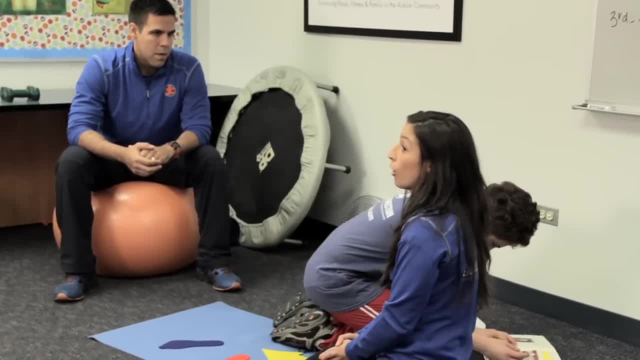 So this is a picture of Dylan exercising, And because he's so motivated by music, he also gets a surprise of one of the musicians or artists that I know of. So this is a picture of Dylan exercising, And because he's so motivated by music, he also gets a surprise of one of the musicians. 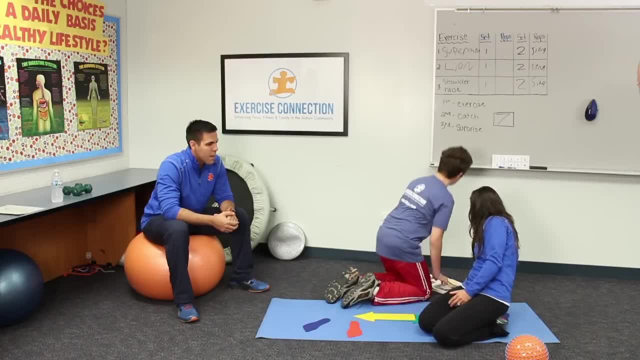 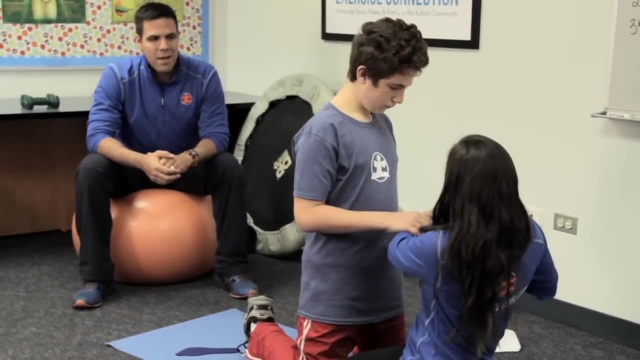 or artists that I know, of Which I just want to show everyone. Who is this? Oh, Sebastian Bach, Sebastian Bach, Very good, Very good. Who is this? Mozart, Mozart, Beethoven, Beethoven, The Three Stooges, The Three Stooges And One Direction.